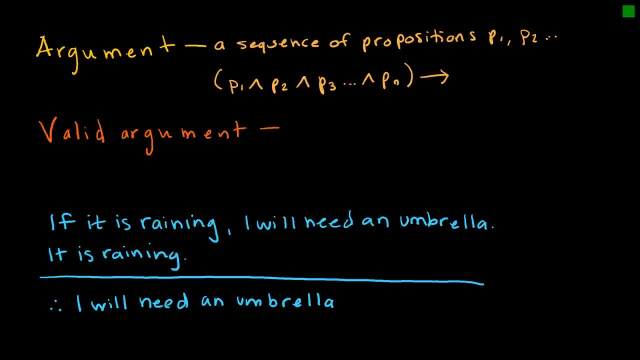 be implies, or if, then Q. So we call P1,, P2, etc. the premises and we call Q the conclusion. And if it's a valid argument, a valid argument would mean that the premises imply the conclusion. Essentially, we're saying: if this is a tautology, it is a valid argument. So if 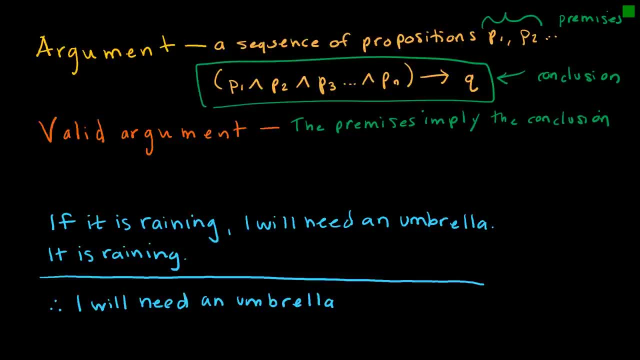 it is always true, then it is a valid argument. So let's take a look at our statement: If it is raining, I will need an umbrella. Then we say it is raining, And let's talk about how we might write this using. 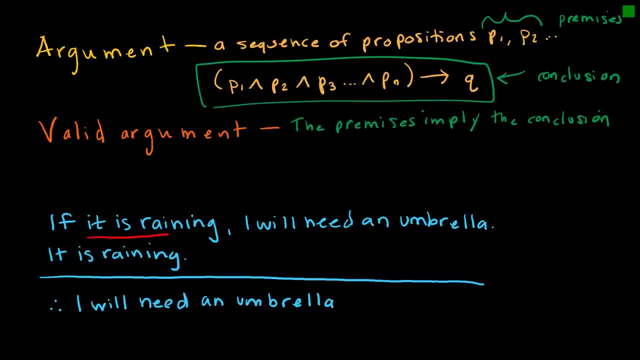 propositions. So let's let it is raining be represented by P. Therefore, this is P, And let's let I will need an umbrella be represented by Q. And here we have an umbrella, And here we have an if-then statement, even though I didn't write the n. 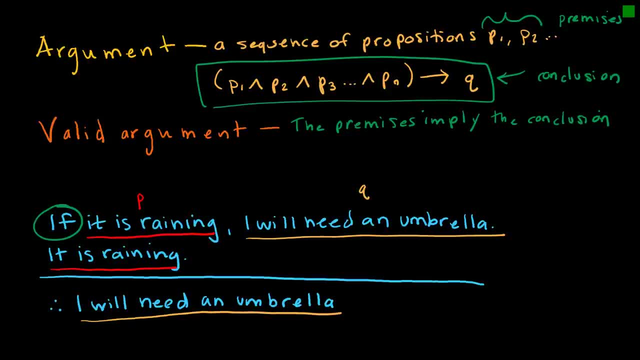 So let's talk about how we would write this. My first statement says: if p, then q. My second statement says: it is raining, so that's p. So we know in our first statement, if p, then q would mean that if p is true. therefore, 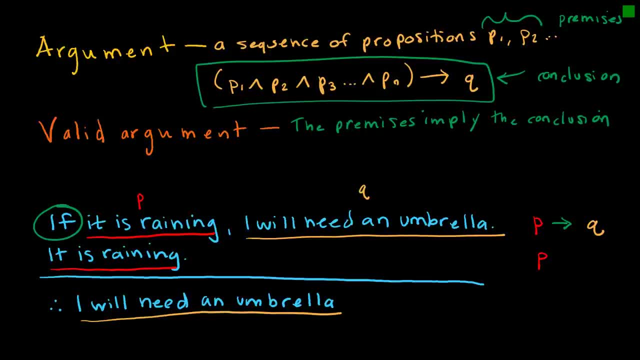 q is true, And then I tell you in the second line that p is true. Therefore, what is my conclusion? And again, remember, the three dots mean therefore: So therefore, we can say q is true. I will need an umbrella Over the next several slides. 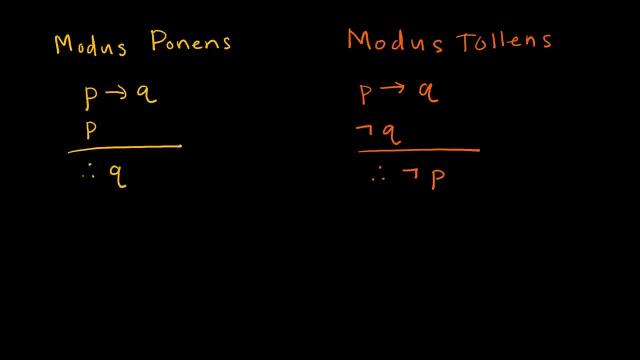 we're going to talk about how to write an umbrella. We're going to take a look at some different rules of inference that we're going to be using, and I'm just going to introduce a lot of them to you and hopefully help them make. 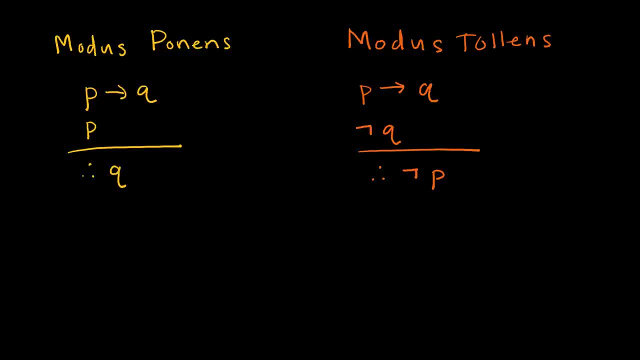 sense to you, so that when we use them you're just ready to go. So we're just sort of building that toolkit for down the road. The first rule of inference is modus ponens, and this should look familiar because we just did an example with the rain and the umbrella on the last slide. 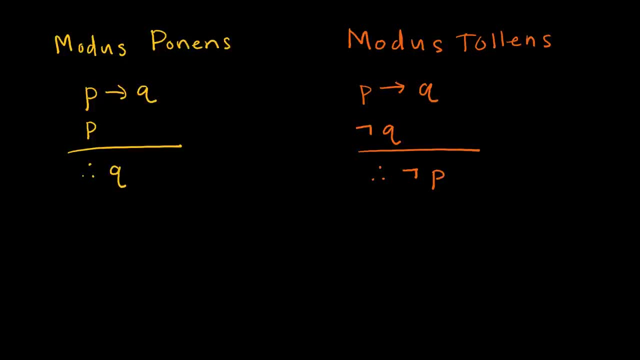 So modus ponens says this: if we have, if p, then q, and then I tell you: p is true, the result is q, And again, this means therefore: So those three dots mean therefore: Now again, this is exactly what we just did. 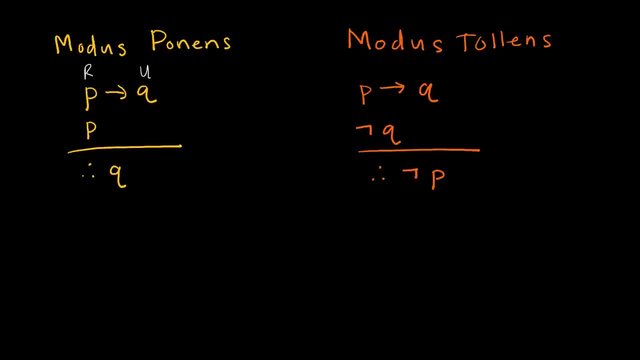 If it rains, then I'll need my umbrella. It rains, therefore I need my umbrella. Great, So how am I going to write this in another way? Because on each of these, we're going to look at how to write them as a tautology. 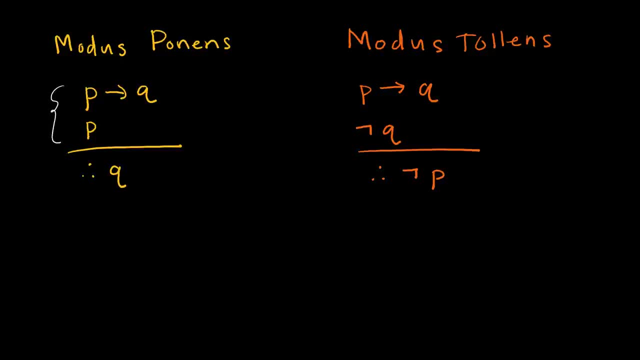 And basically what we're going to do is we're going to say: if this is true, then that's my conclusion. So how would I write all of that stuff on the top? I would say, if p, then q and p. So I'm saying, if this is true, then q is true. 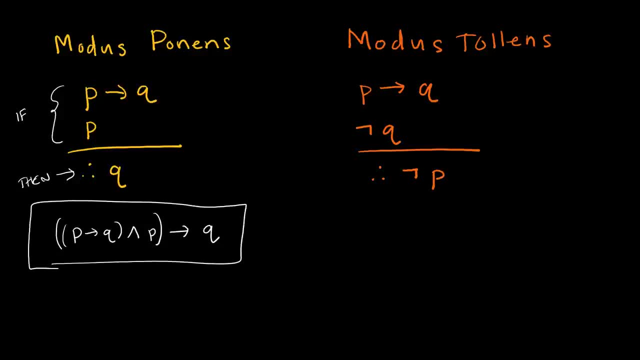 So that's how I would write it as a tautology. Now let's take a look at modus tollens. Very similar: The first statement is the same, The second statement is not q and the result or conclusion is not p. 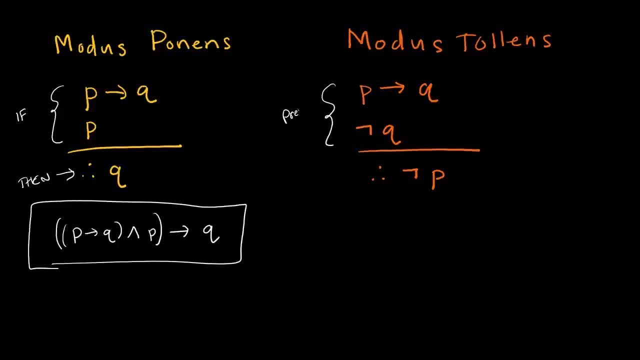 So again, here are the premises, and then, of course, our conclusion, And then a lot of people struggle with this one, just kind of making it make sense in their head. But what I would encourage you to do is think about If p then q, and know that I can write if p then q as an equivalent statement, as if: 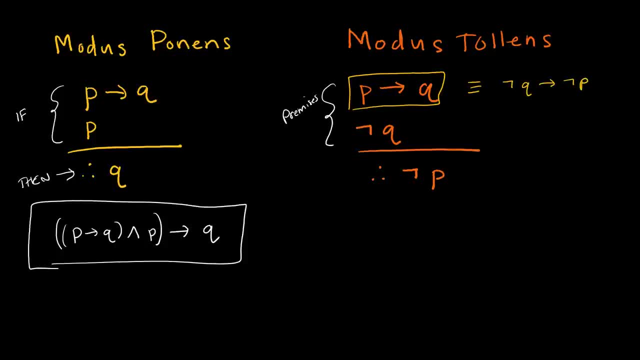 not q, then not p. And to me that makes a lot more sense because if not q, then not p looks exactly like modus ponens. We're saying: if something, then something else, then the first thing is true, then the second thing is the result. 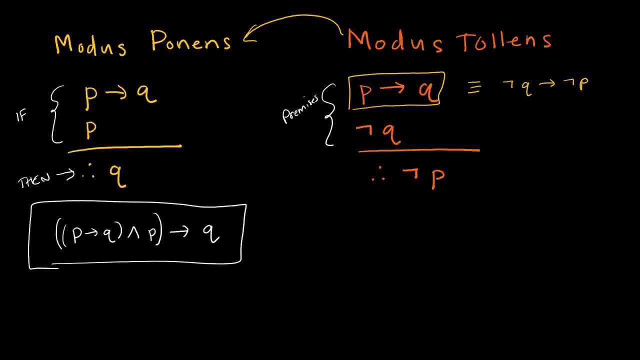 And that's exactly what modus tollens tells us. Now how would I write it? as a tautology, I would write, just as I did before, the premises as the if part of the implication. So if p and q, I'm sorry, if p, then q and not q. if all of that, then not p. 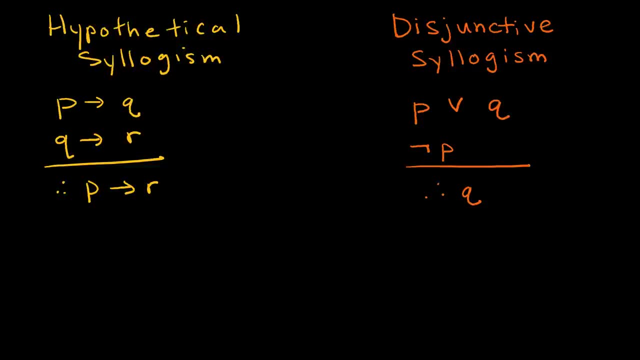 Let's take a look at a few more rules of inference. The first is the hypothetical syllogism, And this is should look pretty familiar. It's very similar to the transitive property. The transitive property says: if a implies b and b implies c, then a implies c. 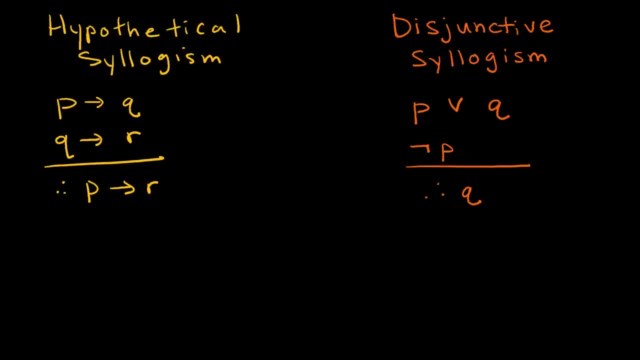 And that's exactly what this is saying. It's saying: if p implies q, so if it rains, then I'll need an umbrella. and then if q implies something else, so if I need an umbrella, then maybe I should wear galoshes. then the 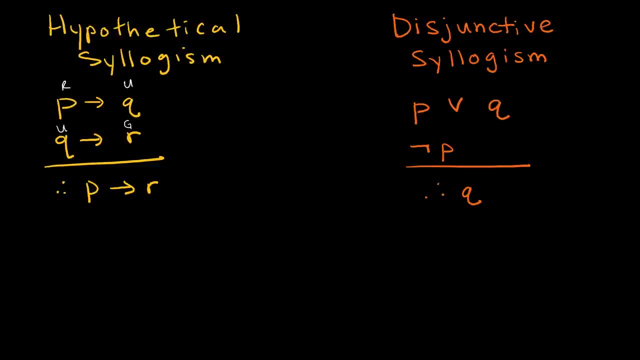 conclusion is: If p, then r, or if it rains, then I should wear galoshes. So that's all it's telling us. is that one implication essentially leads to another. So how would I write that? as a tautology, Again, I'm writing my premises as: if p, then q, and if q then r. and then I'm saying: if 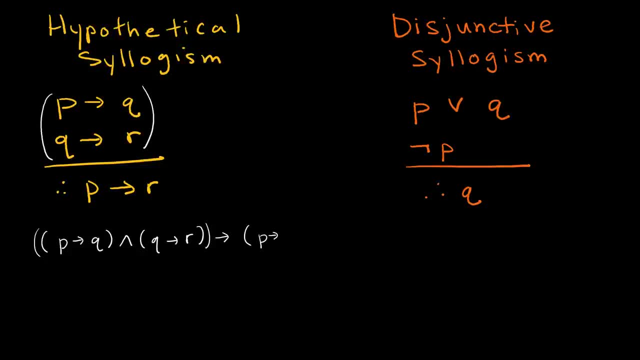 that's true, Then the result is: if p, then r- Hypothetical syllogism. Then we have the disjunctive syllogism again, because this is a disjunction And we're saying p or q and then not p. 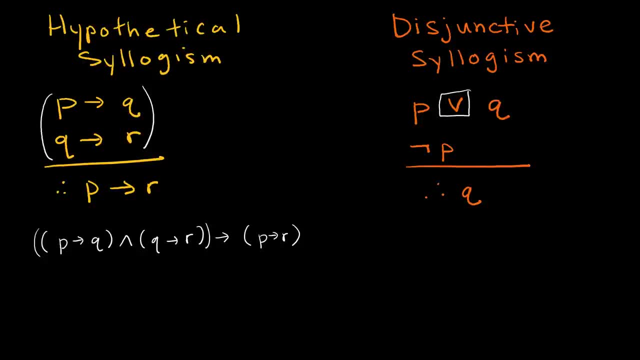 So we're saying p or q occurred, but it wasn't p, therefore it was q. So again, this one makes a heck of a lot of sense to me, Because if we're saying that p or q must have been a tautology, 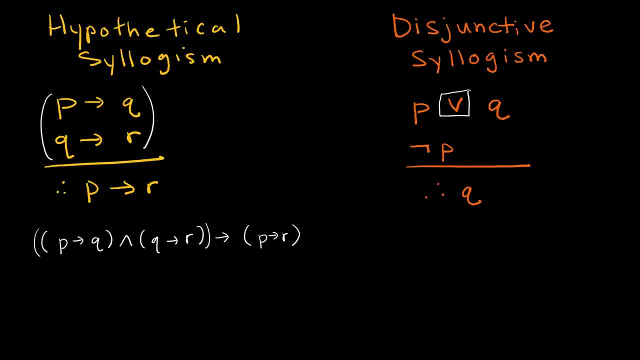 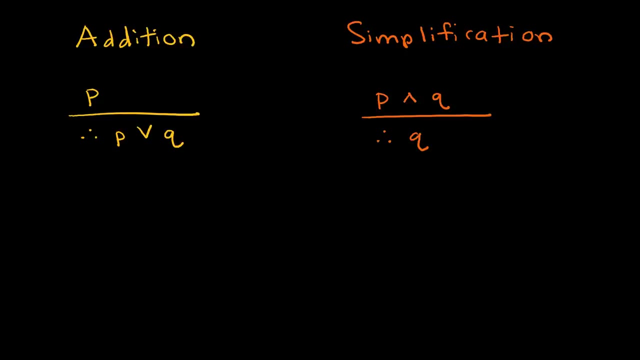 Or q must have occurred, but p didn't occur. it makes sense: q must have occurred. So how would I write that then I would say p or q and not p implies q. The next two rules of inference are kind of silly actually. 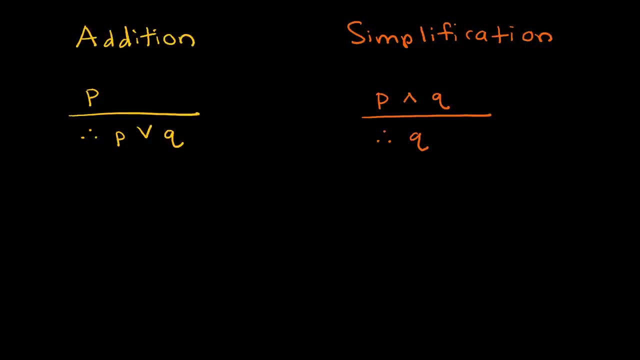 But again, we will use these quite often, but the logic is very easy to follow on these. The first one is addition, and the rule for addition says p, So p is true. is what this is saying. That's the premise is that p is true. 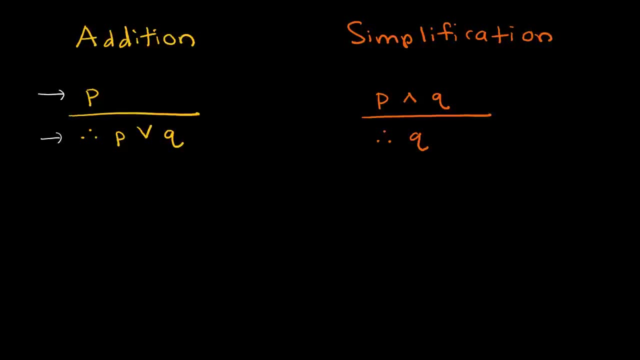 The conclusion is that p or q is true. Well, now this should make sense. We know that when we're dealing with this disjunction with this or statement, that that tells us that one or the other must be true or both. Okay, 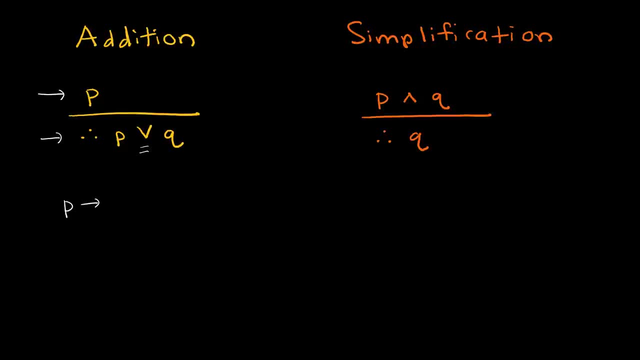 Therefore it makes perfect sense that if P, then P or Q, which is how I would write that as a corresponding tautology. So if P, then P or Q is true, which makes perfect sense. Simplification is the same thing, but kind of backwards. 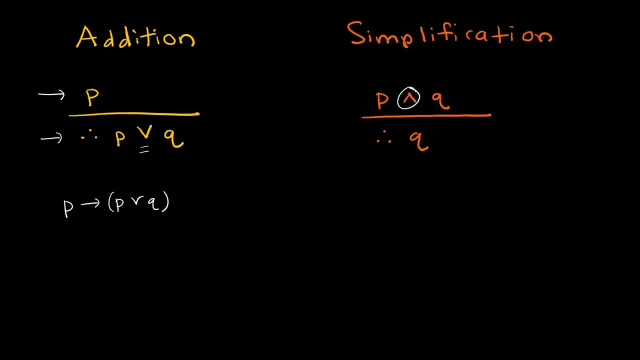 And notice, here we're dealing with a conjunction we're dealing with, and So the premise is that P and Q is true. So let's remember that this tells us that both P and Q are true. So the conclusion that tells us that Q is true is sort of a duh. 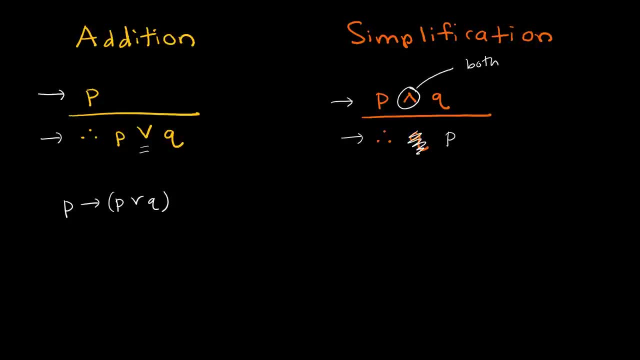 And again I could have: instead of using Q, I could use P instead, And it's the exact same rule. So again, how would I write that? as a tautology? P and Q. So if P and Q, then P, or if P and Q. 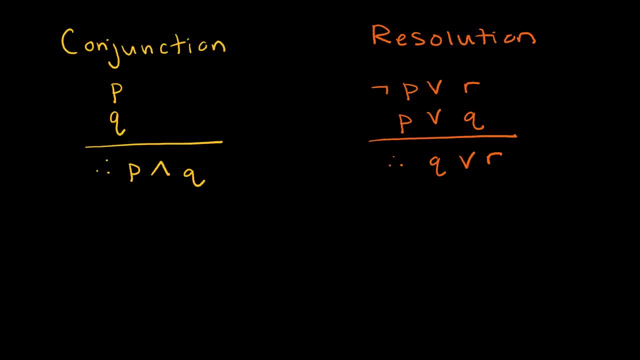 Then Q. both of those would be the same. Let's take a look at our last two rules, the conjunction and the resolution. Now, the conjunction is super straightforward and kind of silly, but really it's just a reminder. Conjunction, which is, of course, what this is says. the premises are that P is true and Q is true. 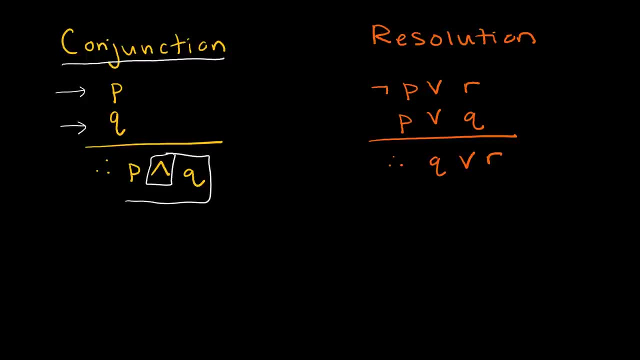 And because P is Q and Q is true, then P and Q is also true, which again we kind of already knew. But that's fine, That's okay. P and Q, So if those are both true, then P and Q, the conjunction is true. 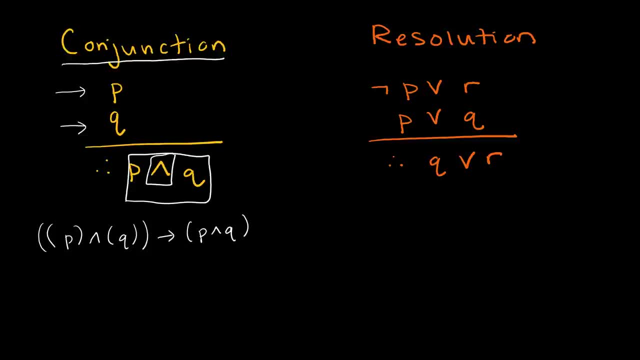 So pretty straightforward and kind of silly, but it gives us a name to use when we're working with proofs. And then, of course, the resolution. Now, this one's probably the hardest one to get your mind around. Resolution is saying that not P or R is true. 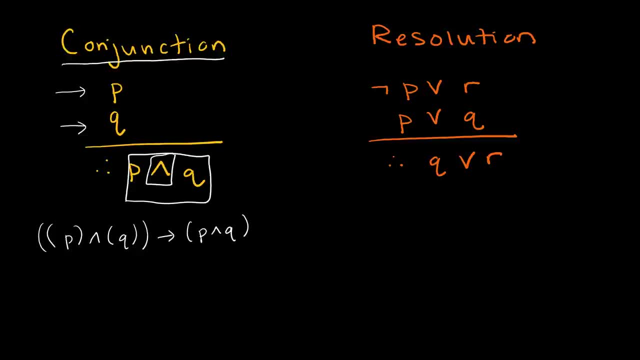 And P or Q is true, And if that's the case, then either Q or R is true or both. So let's think of it this way. Let's pretend not P is true. So if not P is true, then P is false. 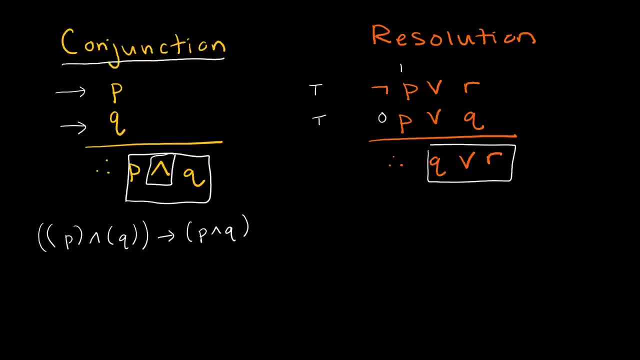 Now for both of these statements to be true, which is what the premise says, that would mean Q would have to be true And R could be true or false, and we don't really care, But because Q is true, that would make this conclusion true. because Q is true. 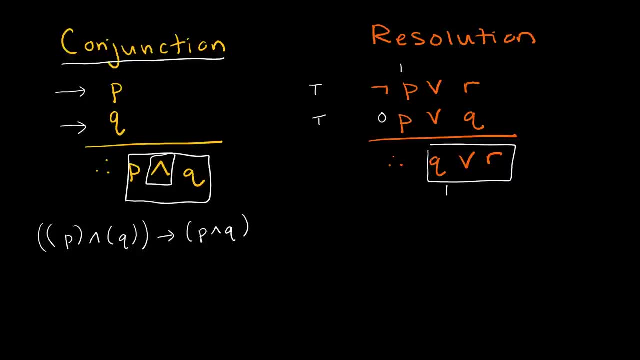 So let's now take a look at: if I changed things up and I said P was true, so not, P was false. So if not P is false, that means R would have to be true for this to be true. And then if R is true, then R would have to be true for this to be true. 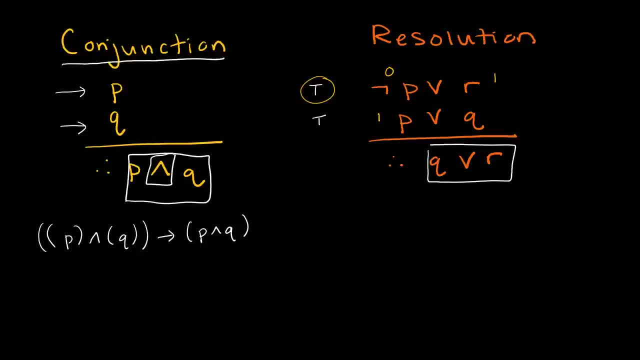 And if R is true, we don't really care if Q is true, because down here I've got a true And therefore no matter what. again, using these premises and the conclusion, we can see that resolution is a valid way of thinking. 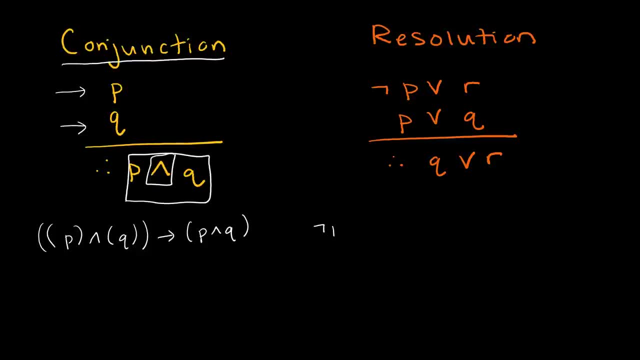 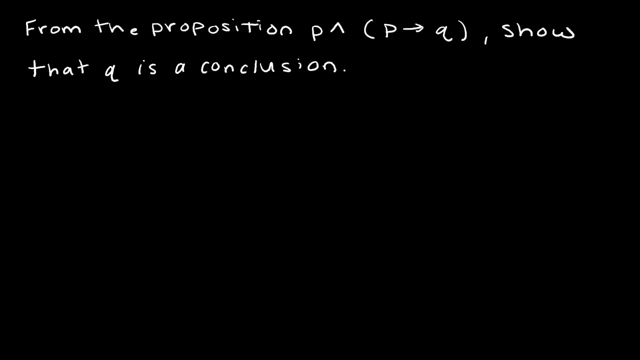 So how would I write that? as a tautology, I would say not P or R and P or Q. So if that, then Q or R. So let's take a look at why we're learning about these. What are these rules of inference for? 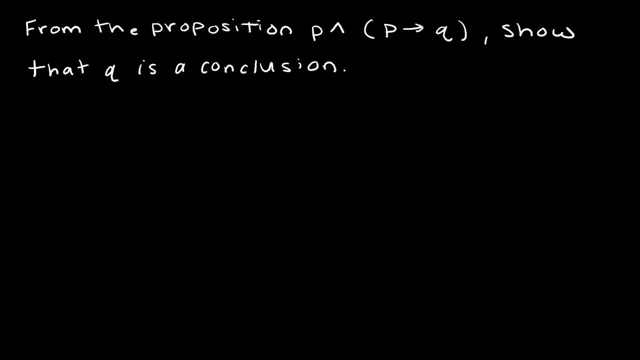 And they are so that we can build a valid argument. And a valid argument says that we're going to be given some information, We're going to be given the premise- and it might be more than one premise- And we need to use those. 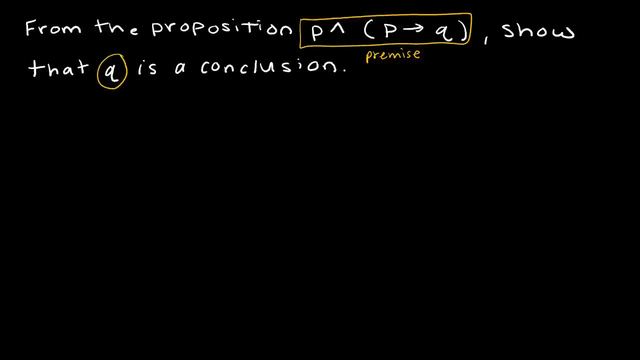 And we need to use those laws to show that some conclusion is true based on the premise and based on the laws. So before we look at this one specifically, let's look at just the general, The general case. we'll start with some reason here. 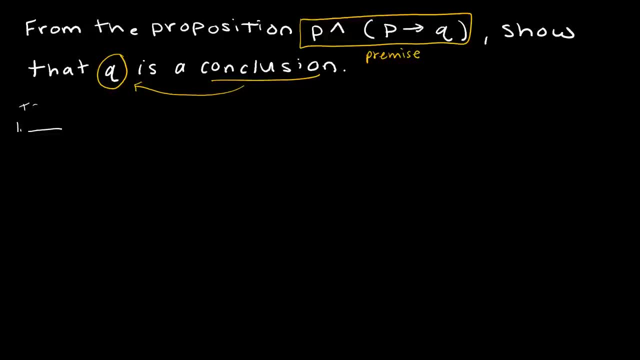 And anything that goes here is going to be a true statement, And then anything that goes here is going to be a reason. So it's going to be like a two-column proof And this, typically the first one- is a premise, And then, from then on, these are going to be your rules of inference that we just learned. 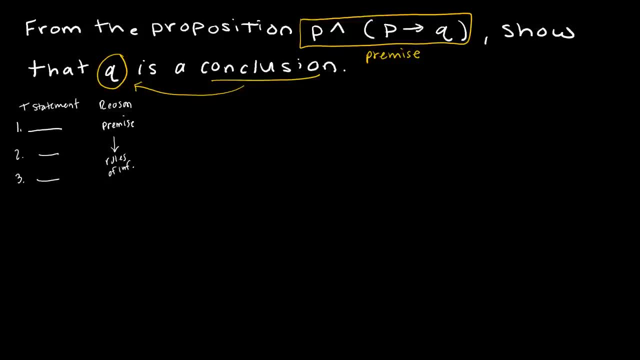 And so I'm going to continue with steps and steps and steps until I get to whatever my final step is. And my final step is going to be my conclusion statement, And the reason again will be some rule of inference, And that's how we're going to build a valid argument. is we're going to say, okay, this is true, because they told me that? 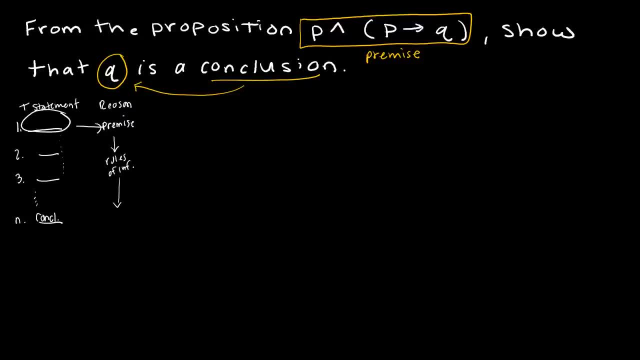 They told me it was true. And then all of these other things are true because of the rules of inference, And therefore this last thing is true, And that's what I wanted to prove was true. So let's put that into action then. 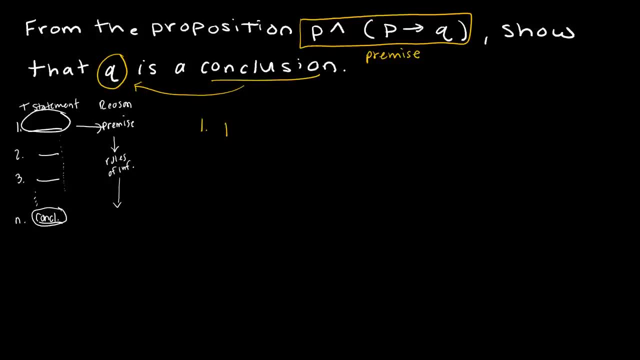 If I were doing this particular question, I would first write P, and if P, then Q, Because I always started out with a premise: Because how else am I going to start? I'm going to start with something that I know I know is true. 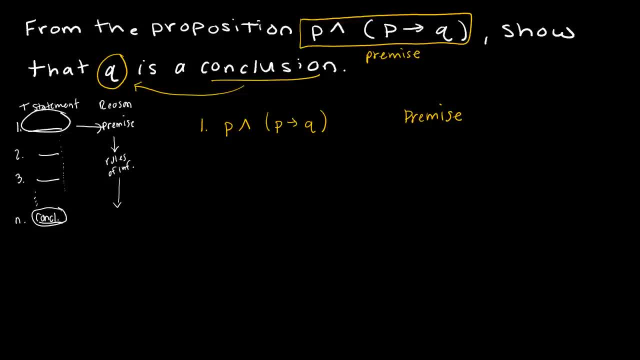 So again P, and if P, then Q is true because they told me it was true. From there I'm going to look at my rules of inference and think about the fact that I'm trying to get to the fact that Q is true. 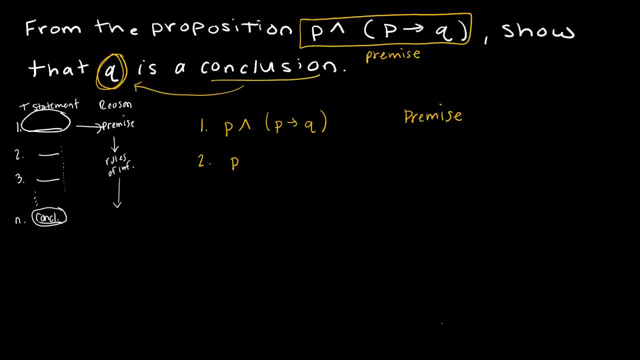 Well, based on my premise, I can say that P is true. And how can I say that P is true? We have a rule, or a rule of inference called simplification, And that simplification Rule says that if you have if P, then Q is- I'm sorry- if P and Q. 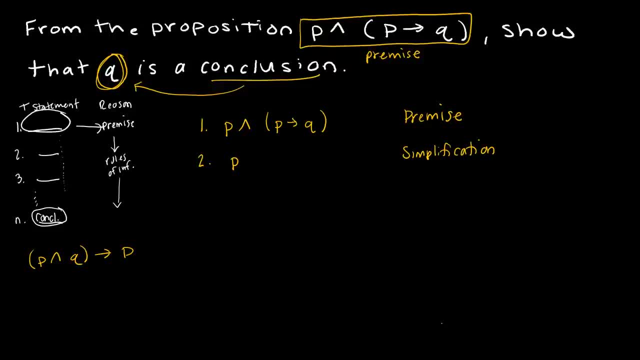 Then P. And it also says if P and Q, then Q, Basically saying if you've got P and Q are true, then P is true, And P and Q are true, then Q is true. So I can say simplification. 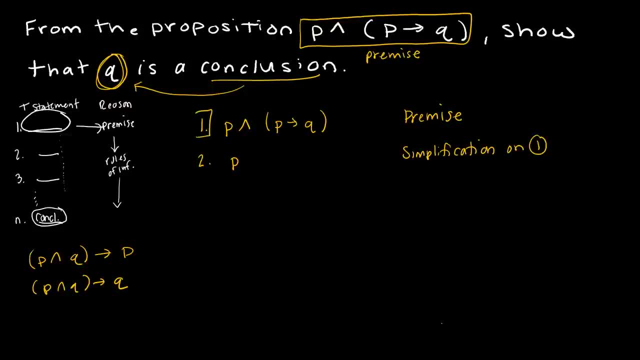 On One. So I'm saying- here's my first statement- I'm simplifying that to say P is true And I'm going to simplify that to say if P, then Q is true. So same reason: Simplification On One. 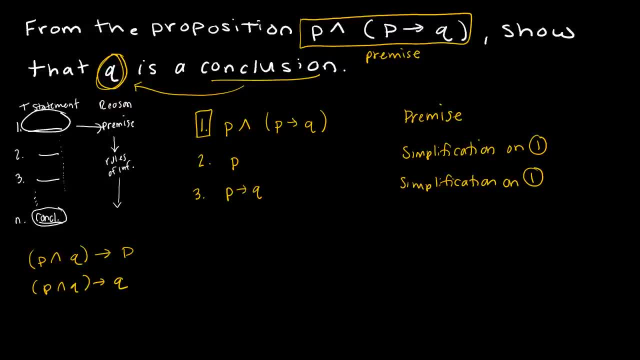 Now that seems silly because I didn't really do anything. I just said two separate statements. But that's exactly what this whole process is about. I'm saying, hey, guess what? This is true Because I can Simplify my first statement. 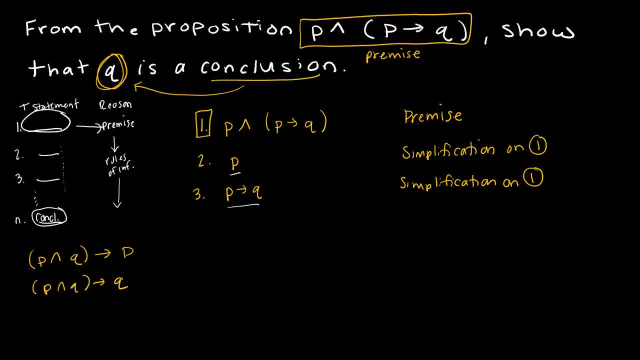 This is true because I can simplify my first statement. My final conclusion is that, therefore, Q is true, And you might be saying, hold up, you didn't really do anything. How did you show that Q is true? Well, we have a rule. 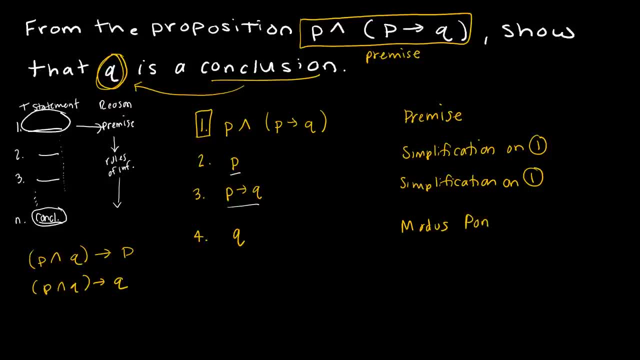 Called modus ponens And if you'll recall- and I'm going to say on two and three before I forget- and if you'll recall, modus ponens tells us That if we have if P, then Q and P therefore Q, and that's exactly what I have here. I have if P, then Q, and I have P and therefore Q is true. 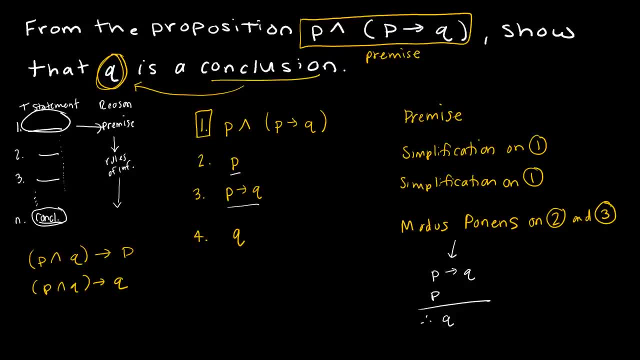 So this is how a valid argument works. I started with a premise that I knew was true, because they told me it was. I used my rules of inference and I got down to my conclusion. So again, here is a premise. Here's my conclusion. 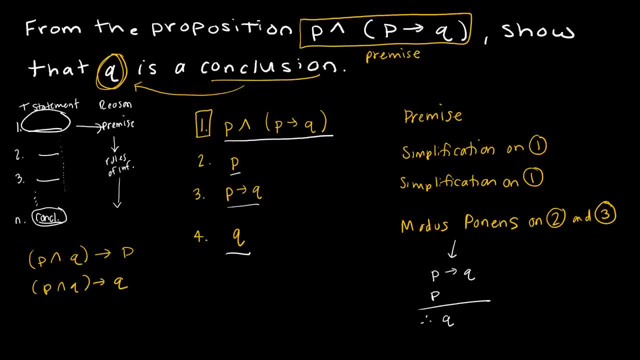 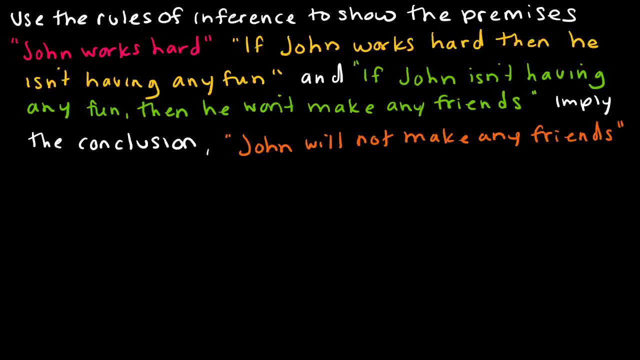 I've shown that that is a valid conclusion. Let's try another example, and this one is going to be harder because we don't know what the propositions are. in the last one it was sort of defined for us, and now we have to define them ourselves, which is fine. 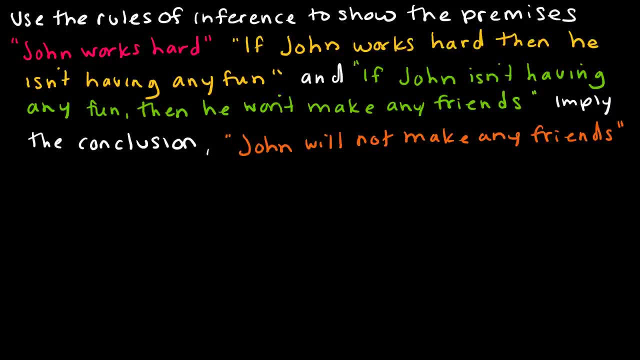 It's just one extra step, So here's how I would get started. It says: we're using the rules of inference to show that the premises John works hard. Okay, so as I'm reading it, I'm just going to say that I'm going to use the rules of inference to show that the premises John works hard. 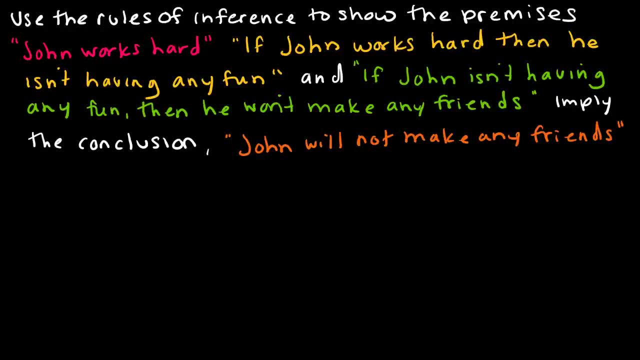 Okay. so as I'm reading it, I'm just going to say that And then he's going to get started for assigning. So I'm going to say that p represents John Works hard. Another premise is: if John works hard, then he isn't having any fun. 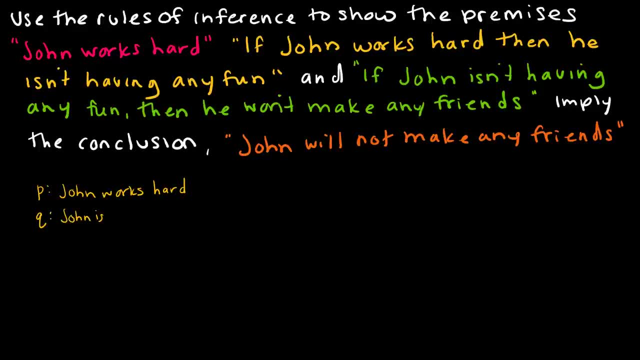 So I'm going to let Q represent John Is having fun, Because I can always negate that when I'm writing the actual proposition, Because I can always negate that when I'm writing the actual proposition. And then if Q represents John Is having fun, then he isn't having any fun. 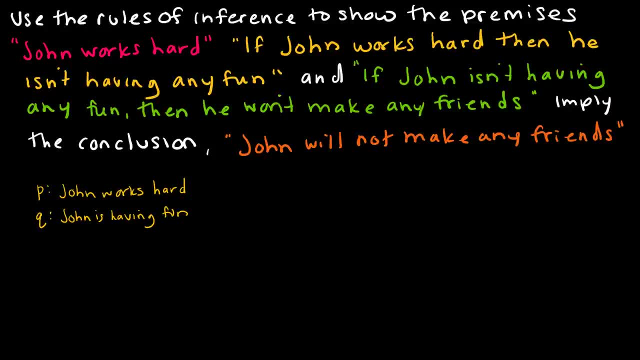 Then if John isn't having any fun, then he won't make any friends. So R is going to be, John is making friends. So this is something you would definitely want to do. before you get started on any sort of logical argument, We need to know what P, Q and R represent. 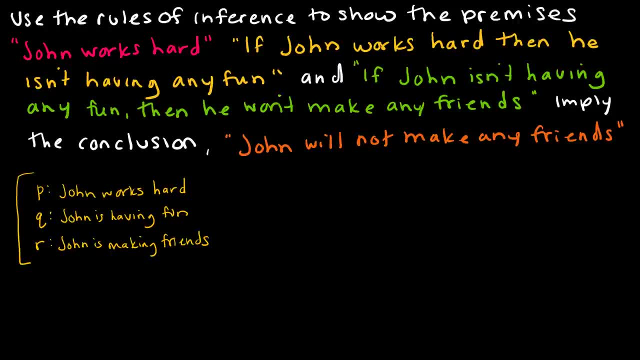 The other thing I would do before I get started is to write down the premises. Oops, P R E M I S E S premises. So the premises are those first three statements. The premises are one. John works hard. 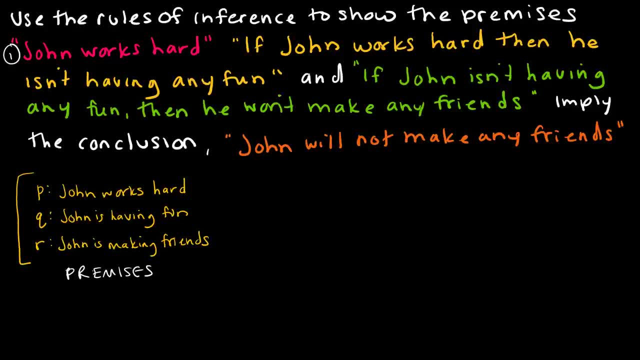 So how could I write that, John? I'm not going to number them or it might get confusing when we do our actual proof. So John works hard is just P Two. if John works hard, then he isn't having any fun, So isn't having fun. 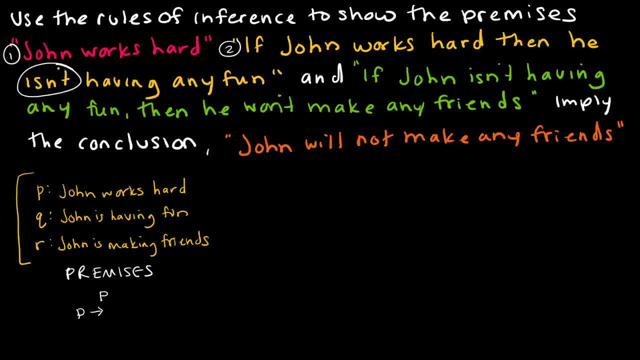 So if John works hard, which is P, if then that's an implication, then he isn't having any fun. John is having fun, is Q, so it's not Q. And then three: if John isn't having any fun, so not Q. John is not having fun, then he won't make any friends. 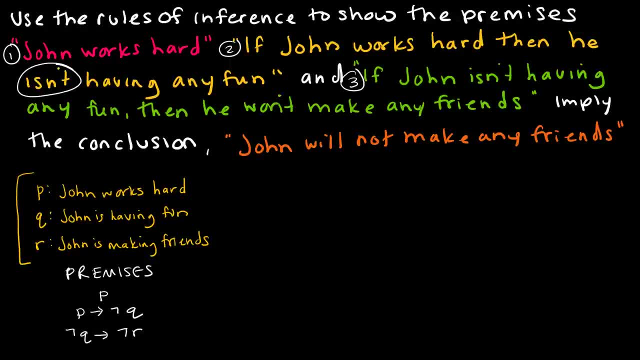 So that would be not R. So these are all premises I can use in my argument, And You'll notice I'm maybe not just going to front load them. So a lot of people like to front load them, And by that I mean they're just going to write all of those things at the beginning. 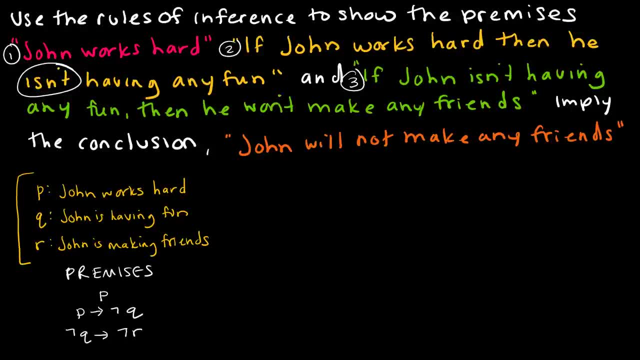 I don't do that because I'm going to write them as I need them Now. the last thing I'm going to do before I get started is I'm going to go ahead and take a look at the conclusion. John will not make any friends. 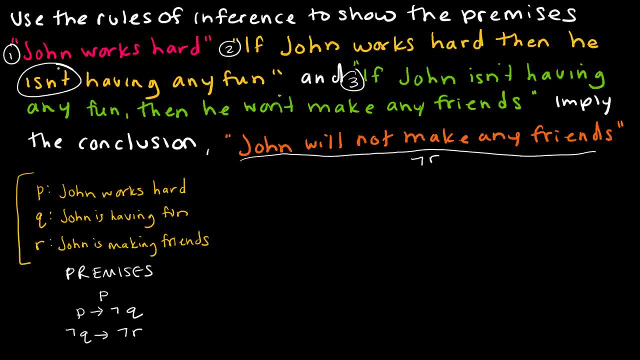 So my conclusion should be not R. Now, it's good to know all of that before I get started, because then I know what I'm going to do, I know what I know, I know what I know and I know what I'm trying to get to. 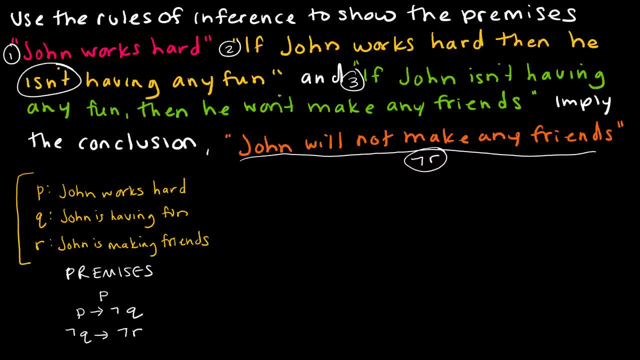 So let's get started now that we are ready. So we had to do a lot of steps to get ready, but now we're ready. So let's go Step number one Again. my first step is really always going to be a premise. 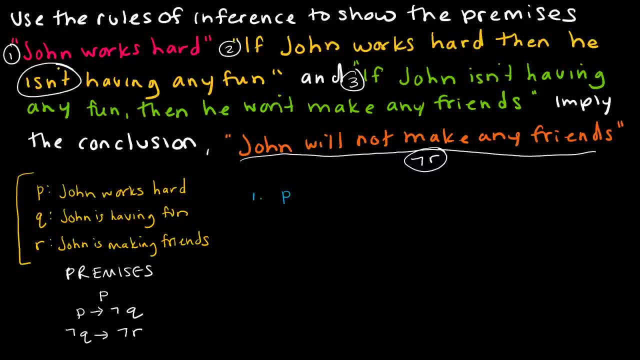 So here I'm going to say P, Because it's a premise. I'm also going to say, If P, then not Q, which is a premise. From here I'm going to use a lot. So notice, I've used this guy and I've used this guy. 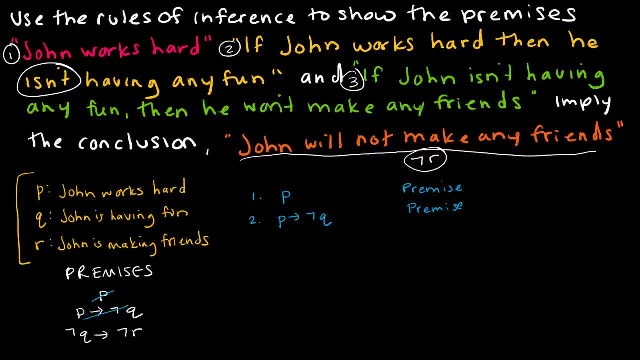 I haven't used the last one yet, and that's okay, because what I'm doing is I'm saying: here's two things that I know to be true, and then here's some conclusion. So if I know, if P, then not Q, and P is true. 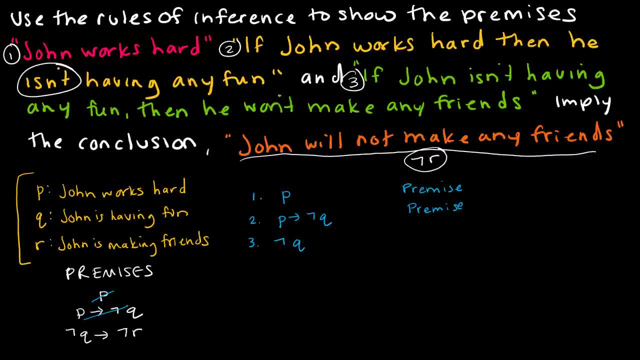 then not Q is true. And that's our good old modus ponens And again, whenever I'm doing a law like that, a rule of inference, I'm going to give the numbers of the statements that I used. So I used the first and the second statement to say that the third statement was true, not Q. 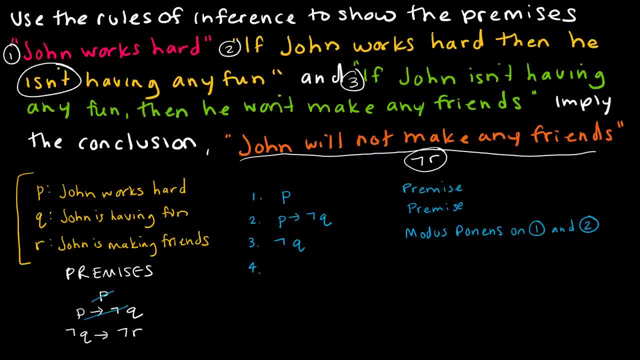 From there I'm now going to say: hey, guess what, If not Q, then not R, And this was a premise. So now I've used that last premise. but notice, I didn't put it at the beginning, I didn't use it until I was ready to. 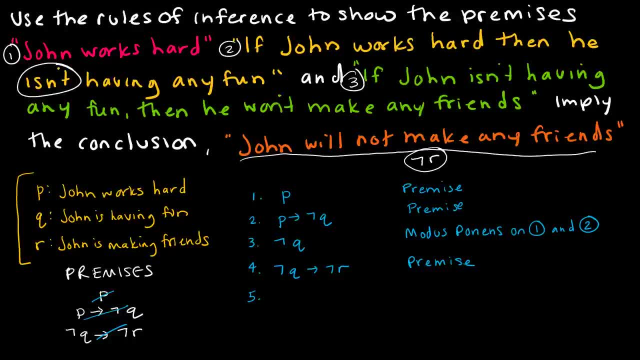 Because now what I can say is, if I have, if not Q, then not R, and I know not Q is true. yep, that's right. I can say not R is true. and the reason I can say not R is true. 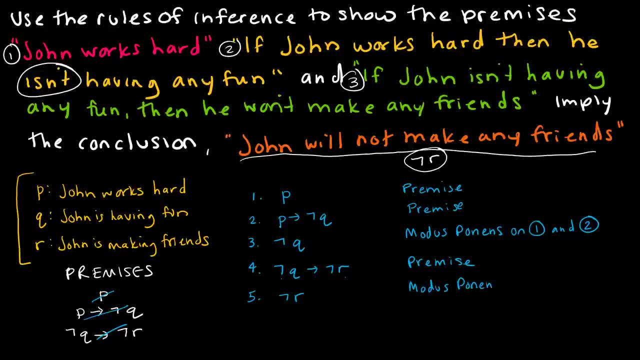 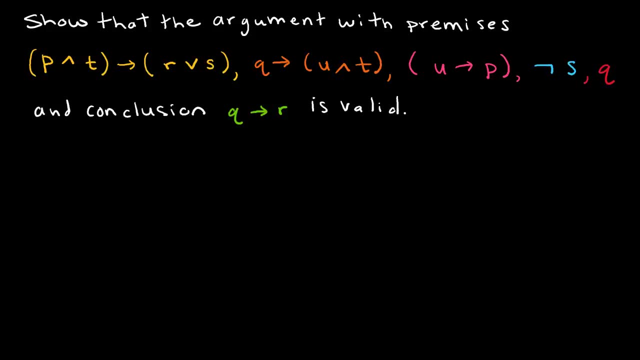 is modus ponens on three and four. And again, that's exactly where I was trying to get to. is that not R, was true? All right, I hope you are ready for this one, because this one is going to be a bit of a doozy. 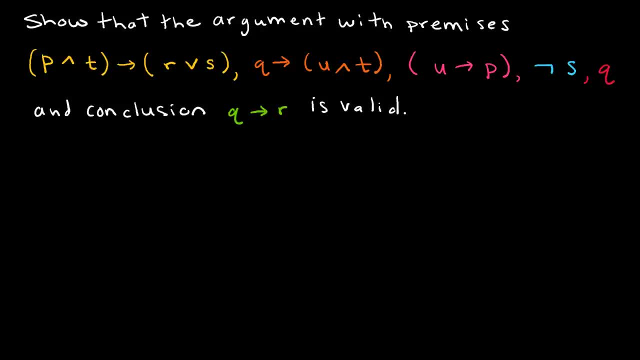 Here we are going to show that the argument with the premises if P and T, then R or S, if Q, then U and T, U implies P not S, Q. These are all premises That those will lead to the conclusion that if Q, then R is valid. 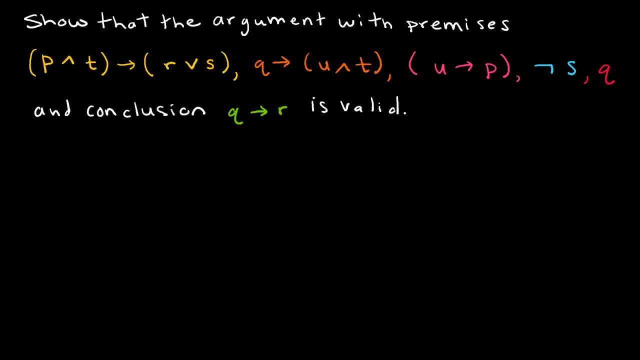 So I know when I start a question like this, it's a little bit overwhelming. What do I know? What do I not know? What am I trying to get to? So, of course, what I'm trying to get to is my conclusion. 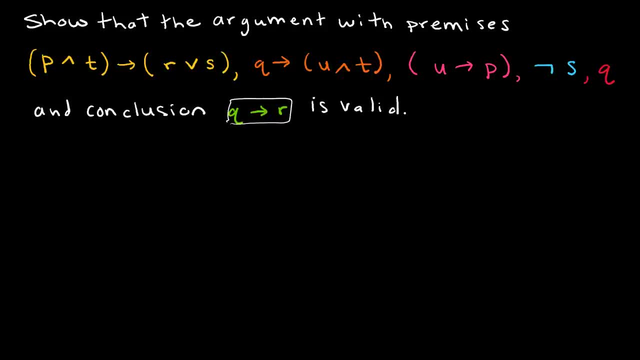 Here's where I'm trying to get, And I've got one, two, three, four, five premises. So right away we know we're going to have quite a few steps in this logical argument. So let's get started together and see how it goes. 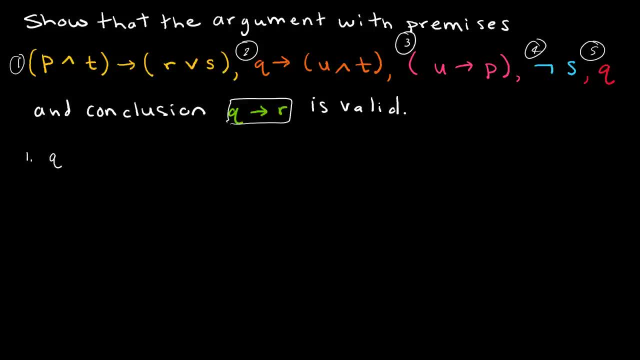 I'm going to start with one and one. I'm just going to say Q, So Q is true because it's a premise. So what else can I say? Well, I'm going to say: if Q, then U and T. 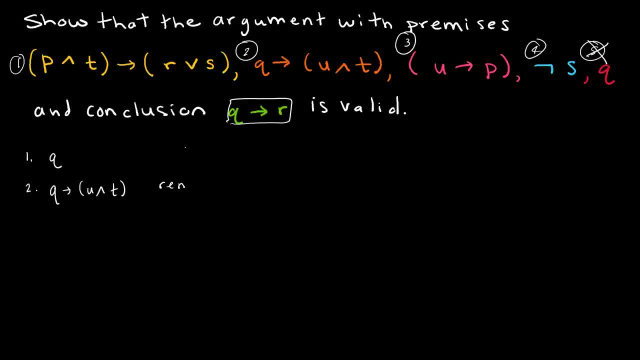 Again a premise. I'm going to move these over a little bit just because I haven't given myself a ton of room. So, premise and premise. So that's this premise and this present premise. I've used both. Now why would I use both of those? 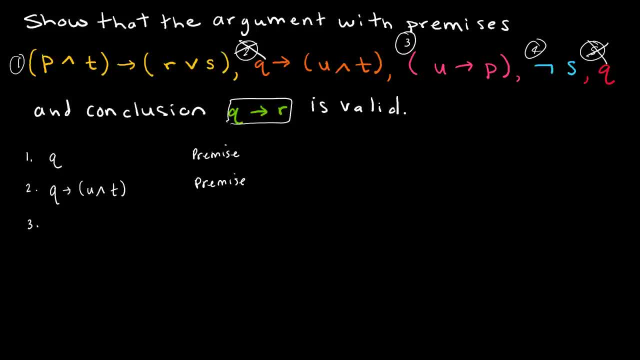 Well, because I know that if Q, then U and T is true, and Q is true. therefore U and T is true. So how do I know that? Yeah, that's right. Modus ponens on one and two. So how does that help me? 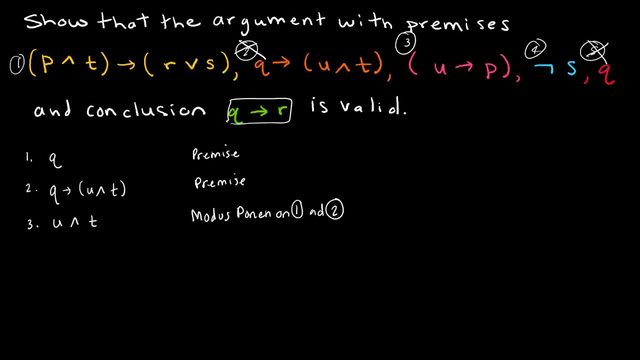 Well, let's think about what I can do next. If I know that U and T are true, then I should be able to say that U is true And I should be able to say that T is true. And I can do that by simplification. on three: 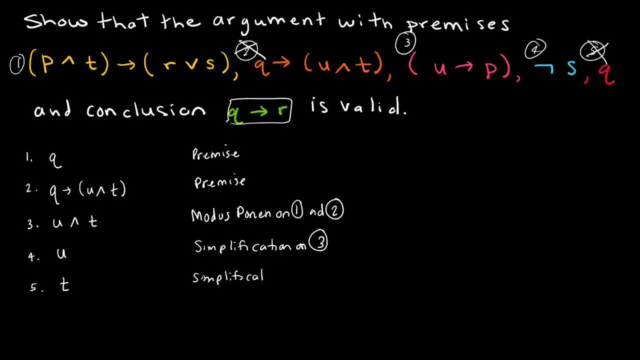 Same here. So now what? Well, I'm going to say that U and T are true, And I'm probably going to take a look at another premise now, because I've sort of gotten to the end of what I can say so far. 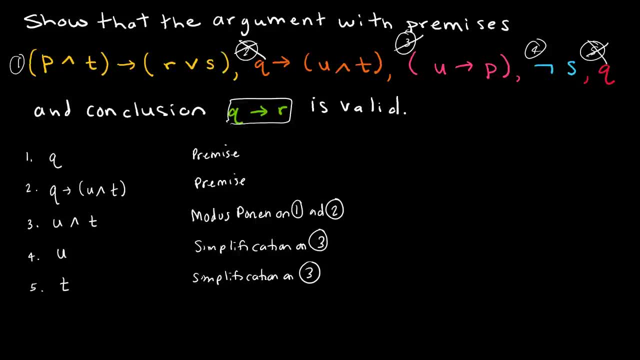 And I have one that says: if U, then P. So let's do that next. If U, then P, And that's a premise. Now why would I need to know that? Well, if I have if U, then P, and U is true, then my next step should be that P is true. 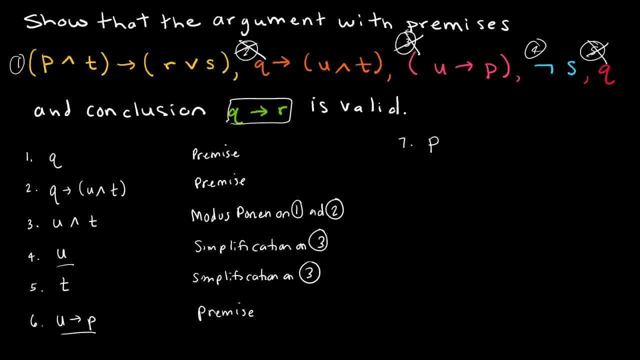 And why is that true? That's modus ponens on five- I'm sorry, four- and six. So P is true. Now think about what I haven't used yet. in my premises I've got P and T. Well, I just showed that P is true. 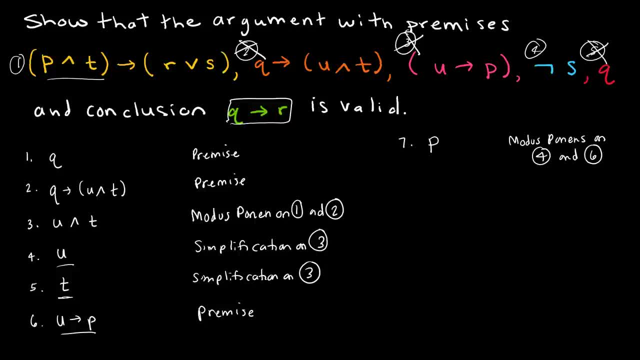 Over here. on step five I showed T was true. So step eight is going to be P and T. I don't really need the parentheses, but you can have them if you want either way. So P and T. And how am I able to show that? 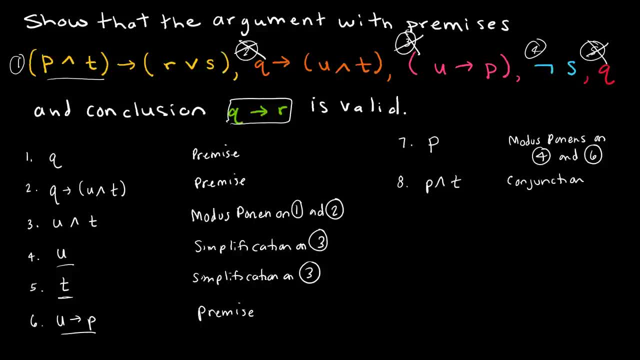 That's a conjunction of five and seven. So now that I've shown P and T, then I can say this premise. So I'm just going to recopy that premise: If P and T, then R or S, And that's a premise. 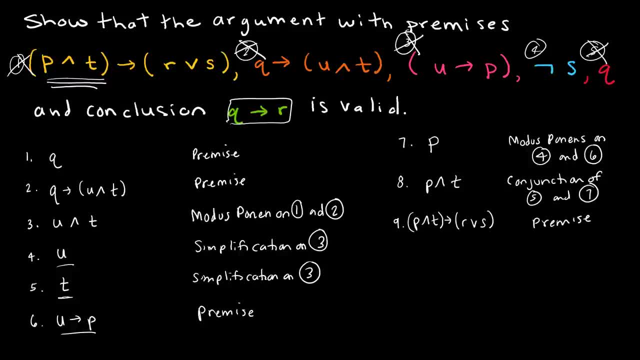 That's a premise. And then for ten, I'm going to say, hey, guess what R or S is true. How do I know R or S is true? Modus ponens. on eight and nine, my pen stopped working for a second. eight and nine.